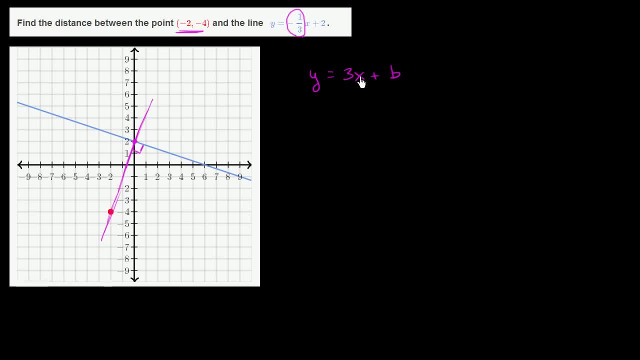 but this point has to sit on it. So this point has to satisfy this equation. So when x is negative 2, y is negative 4.. Or we have: negative 4 is equal to 3 times negative 2 plus b. Let me write the negative 2 in there. 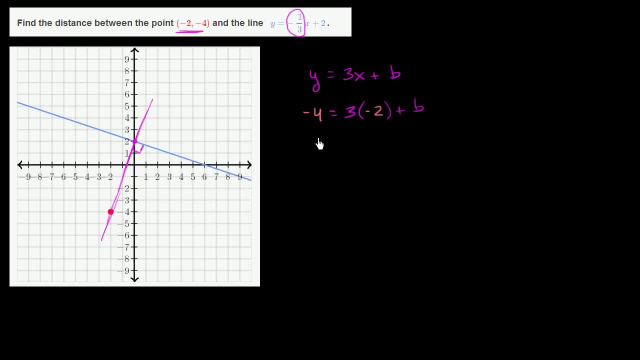 3 times negative, 2 plus b, And now we can solve for b. We get negative. 4 is equal to negative, 6 plus b. Add 6 to both sides, You get 2 is equal to b or b is equal to 2.. 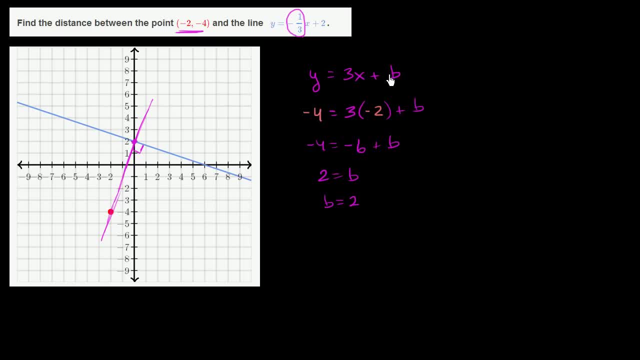 So we were right. The y-intercept for the second line is at 2.. So we immediately can eyeball or we can verify where they both intersect. They both intersect. the y-axis at y equals 2.. For both of these, when x is equal to 0,, y is equal to 2.. 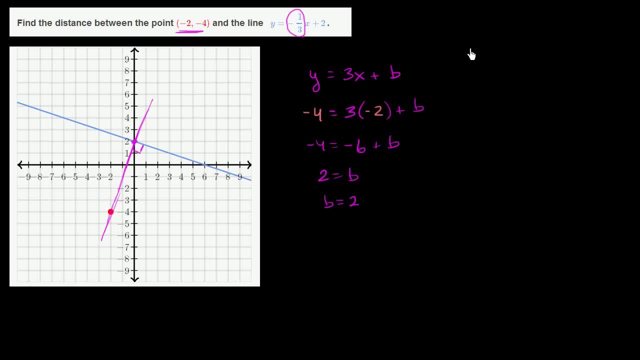 If it wasn't so obvious, we could set these two equations equal to each other. We could say: look, we have 3x plus 2.. We know that this is now 3x plus 2 because b is 2.. 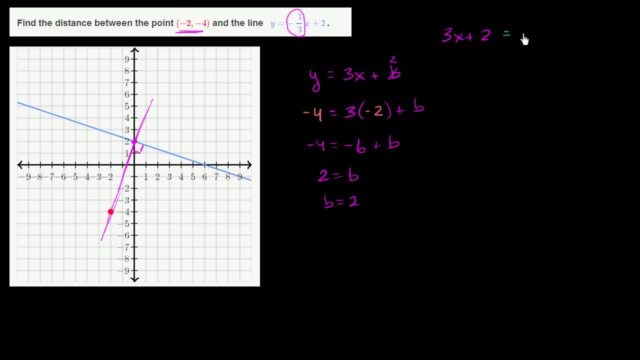 When does 3x plus 2 equal negative 1 third x plus 2?? Well, let's see, If we subtract 2 from both sides, when does 3x equal negative 1 third x? Well, there's a couple of things that we 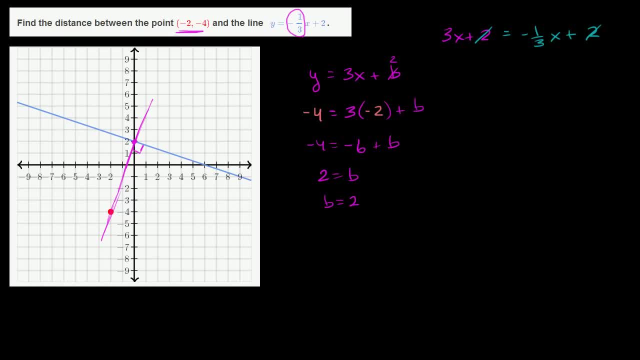 could do right over here. We could add 1 third x to both sides, and then we will get 3 and 1 third, which is the same thing as 10 thirds. x is equal to 0. And if you multiply both sides by 3 tenths, 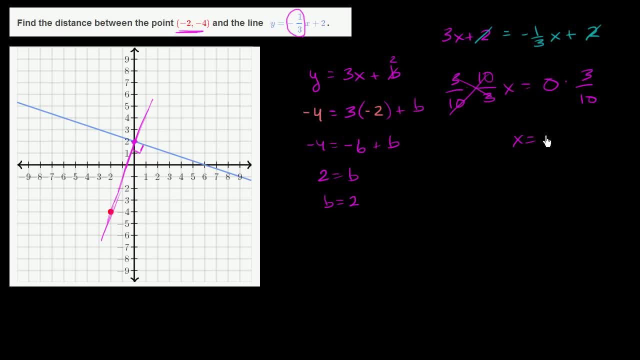 you get: x is equal to 0. So these two lines intersect when x is equal to 0.. For both of them, when x is equal to 0,, y is equal to 2.. But you could have eyeballed it here. 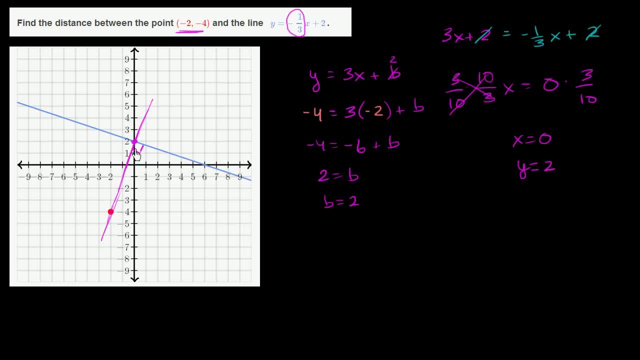 You could have seen that both of their y intercepts, which happens When x is equal to 0,. y is equal to 2.. So this point right over here is the point 0, 2.. We already know that this point right over here. 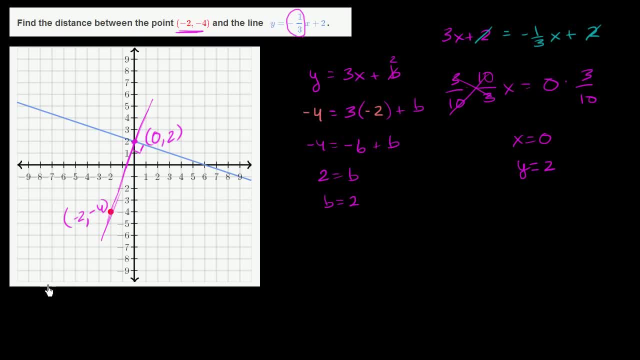 is the point negative 2 comma, negative 4.. And now we just need to find the distance between these two points, And the distance formula really is just an application of the Pythagorean theorem. We just need to find the distance in the change in the y direction and the change. 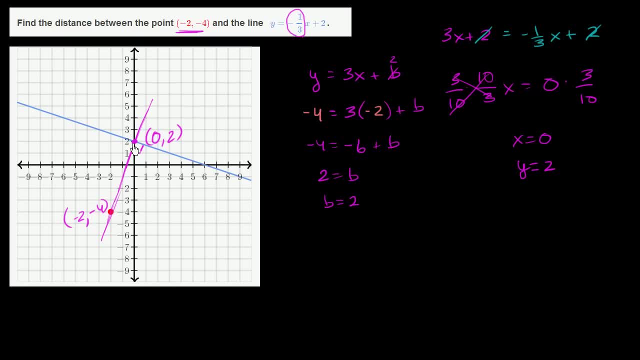 in the x direction, So let's do that separately. So in the y direction, What is this distance right over here? So we went from y is equal to negative 4 to y is equal to 2.. This distance right over here is 6.. 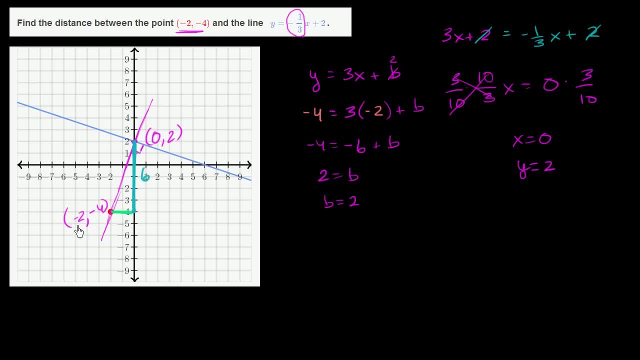 And what is this distance right over here? Well, we go from x equals negative 2 to x equals 0. So this distance right over here is 2.. So the distance between these two points is really just the hypotenuse of a right triangle. that 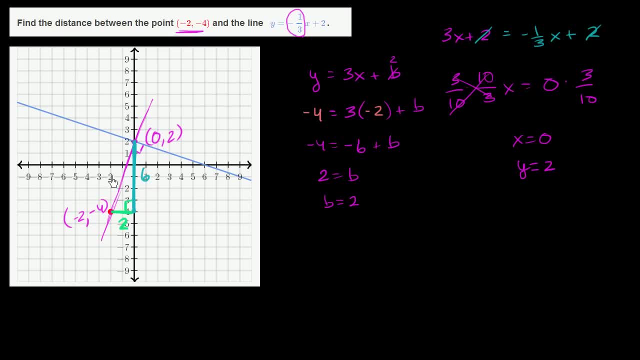 has sides 6 and 2.. So we could say, if we were to do this, we could say: oh well, if we call this distance d, we could say that the distance squared is equal to. And all I'm really doing here is restating the distance formula. 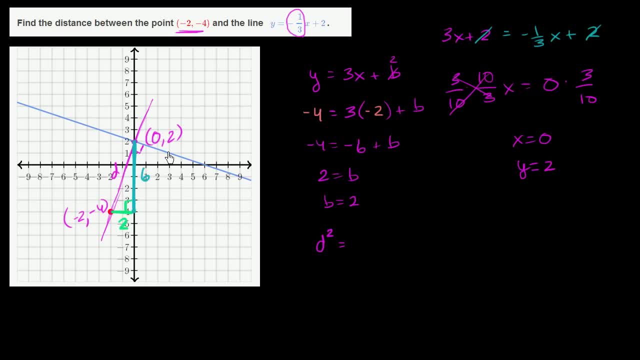 The distance formula tells you all this. you know, y2 minus y1,, which is 6, squared, And that's just the Pythagorean theorem. That's just saying 6 squared plus x2, minus x1, which is 0,, minus negative 2,, which is positive, 2 squared. 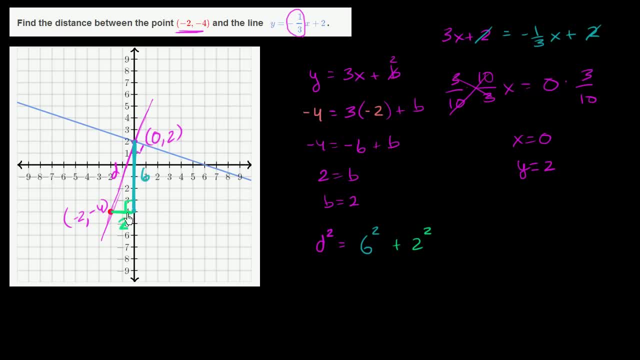 is going to be equal to the distance squared. But we see that's just the Pythagorean theorem. But anyway, let's solve for the distance. So the distance squared is going to be equal to 36 plus 4, which is 40.. 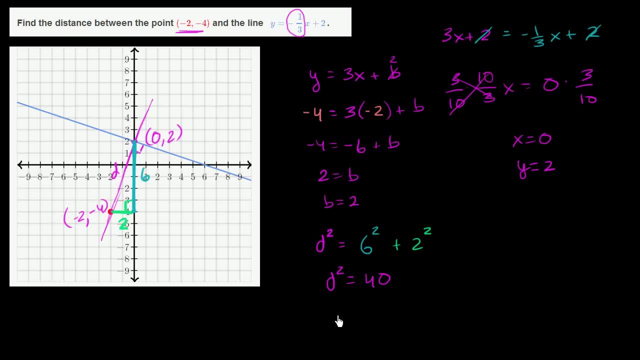 And now we can. let's see 40, so the distance squared, or I could just say the distance, is equal to the square root of 40.. The square root of 40 is the same thing as the square root of 4 times 10.. 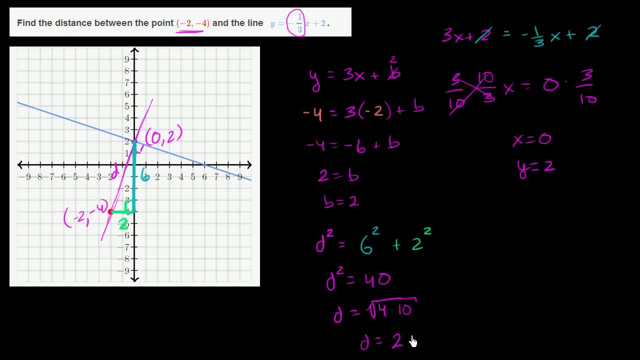 And so that's the same. So the distance is equal to 2.. If we factor out the 4, it's the square root of 4 times the square root of 10.. 2 is the square root of 4.. 2 square roots of 10.. And we're done.